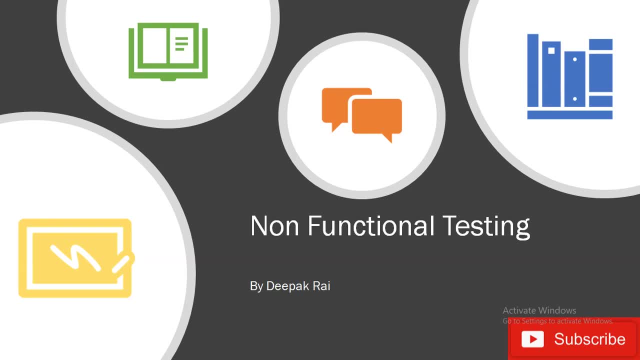 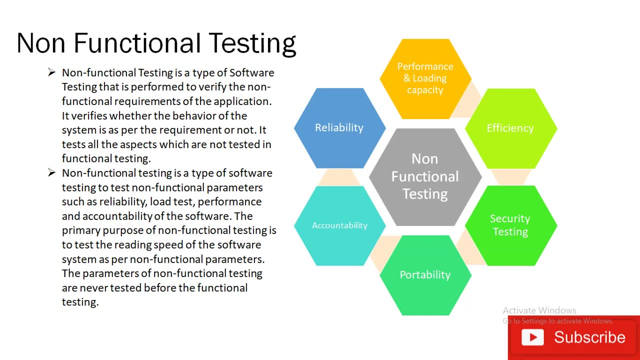 We will discuss about some of the examples as well. Let's start So. first of all, what is non-functional testing? Non-functional testing is the type of software testing that is performed to verify the non-functional requirement of the applications. It verifies whether the behavior of the system is as per the requirement or not. It tests all the aspects which are not tested in the functional testing. 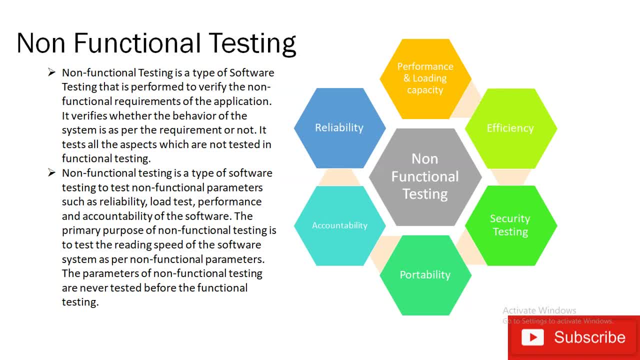 So in my previous session I have already explained about non-functional testing. So let's start with what is non-functional testing and their parameters, where we are using that parameters and what is the types of the non-functional testing. So in my previous session I have already explained about the functional testing and their types. 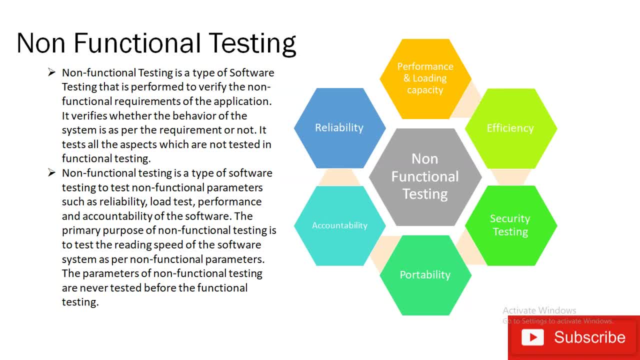 So what ever we have not covered in the functional testing, that thing we are comveryting in non-functional testing. So non-functional testing is the type of software testing such as reliability, load test, performance and accountability of the software. So you can see in this image: 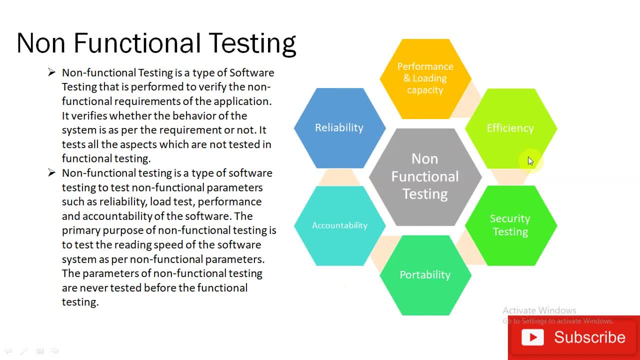 we are checking on the performance and load capability of the computer. performance and load capacity, efficiency, security testing, portability, accountability and reliability of the applications. There are several other terms which are also used in the non-functional testing, like configuration testing. then there is a compliance testing. 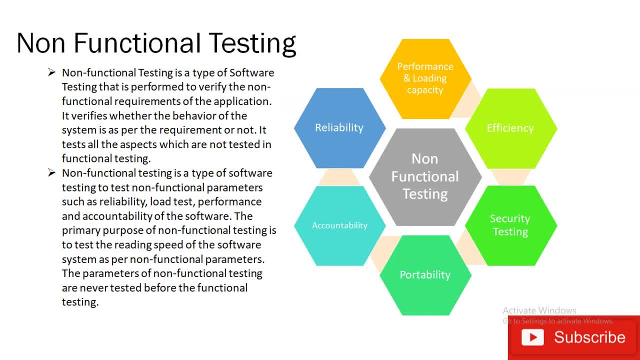 then volume testing. These are also a part of the non-functional testing, But majorly this is considered so volume testing will be covered in the performance and load testing. So the primary purpose of the non-functional testing is to test the reading speed of the. 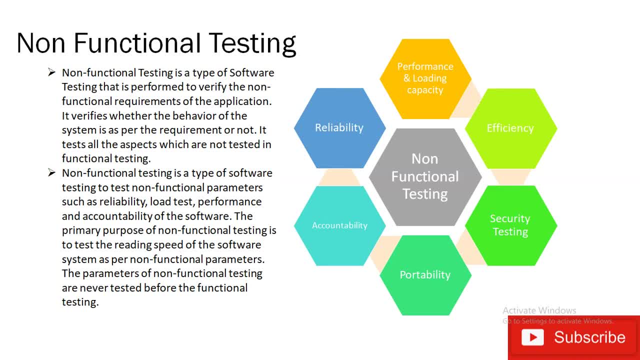 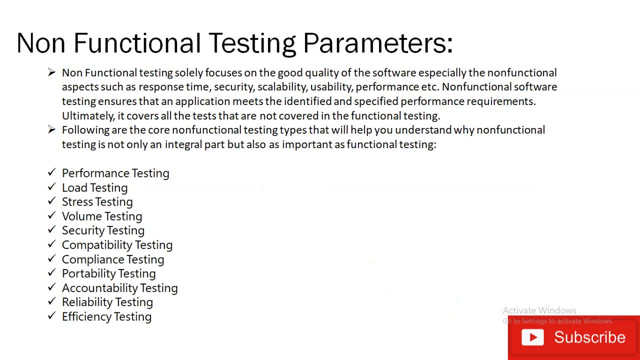 software system as per non-functional parameters. The parameters of non-functional testings are never tested before the functional testing. So what? all parameters are involved in the non-functional testing we will discuss here. Non-functional testing solely focuses on the good quality of the software, especially non-functional 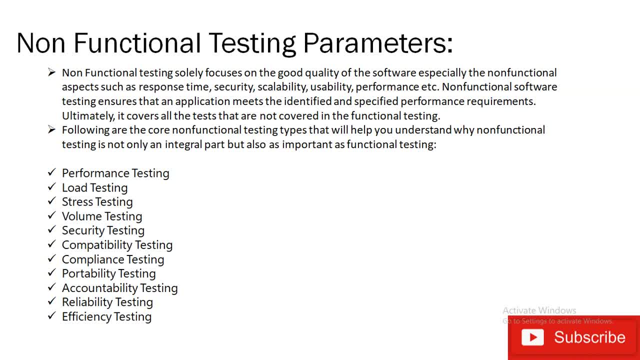 aspects such as response time, security, scalability, usability, performance, etc. Non-functional software testing ensures that an application meets the identified and specified performance requirements. Ultimately, it covers all the tests that are not covered in the functional testing. So, just like, if I want to check the performance of the any website, how it is performing when, 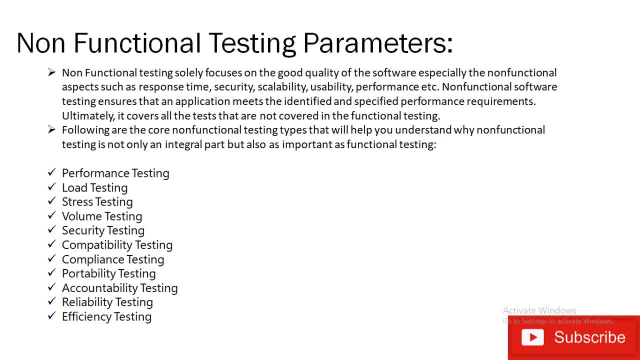 multiple users or millions of users are interacting at the same time. So just like if you are taking any example of the Flipkart application at the time of mega sales offer, So that mega sales offer is that application responding correctly and the response time is proper to the user. 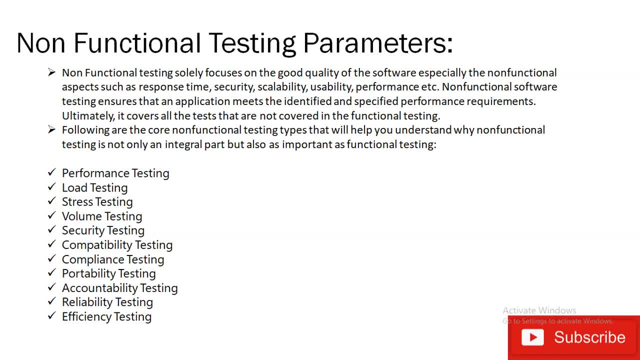 So that user can Add any product in their cart or User can buy any product from start to end of the procedure, just like adding or Selecting the address, then after selecting and in the payment method after payment, better if they want to transfer the amount. 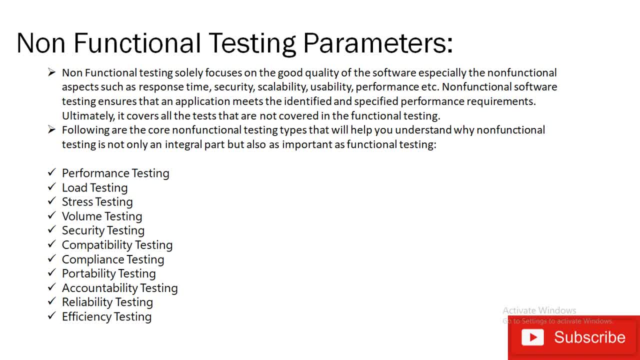 Through net banking or any other channels that should work In a given time period Or it should be in an efficient way to provide the response. There are some core functional testing types that will help us to understand why non-functional testing is not only an integral part, but also as important as functional testing. 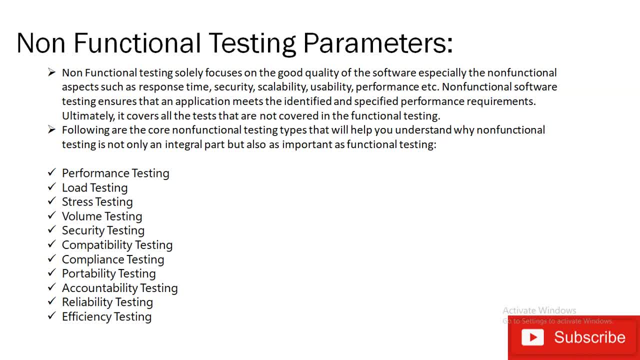 So, in functional testing, we are checking the actual functionality of the application, but non-functional testing is also required In terms of performance. In terms of performance In terms of load, in terms of stress, volume, security, compatibility, just like if we are. 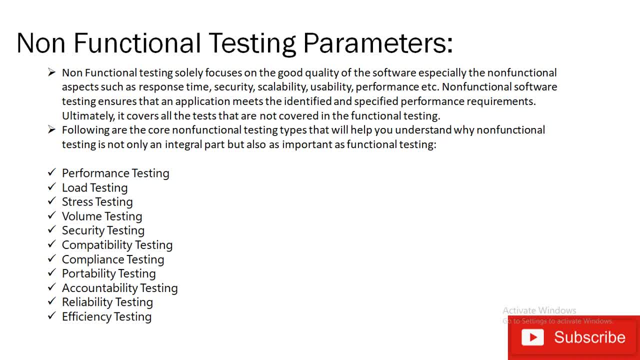 taking up any example of any website, and that website is working in Internet Explorer and theme website is unable to launch in Google Chrome. So that is a major drawbacks as, in terms of compatibility, So it is not compatible to Google Chrome. So, anyway, That has been a big point. 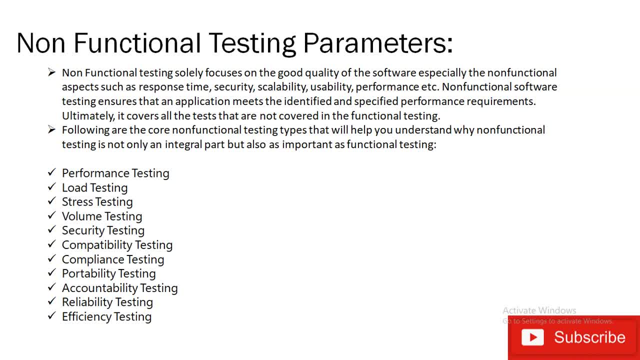 You should work in any of the browser, because we don't know user is using which browser. so if application is able to open in the Internet Explorer but user is using a user is opening that same website in Google Chrome and it is not working, Then user may not try it again to use that website because many of the user is not using. 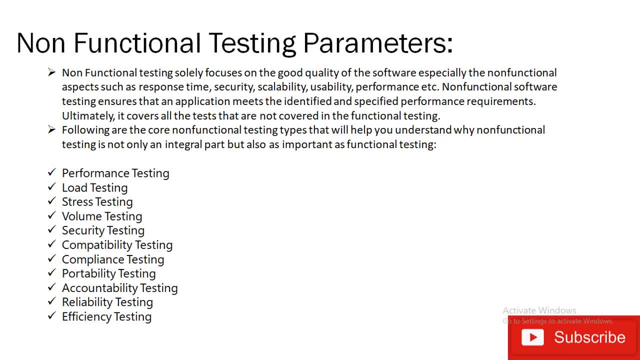 Internet Explorer, many of the using Internet Explorer as well, And some of the users are trying to not using web. They are trying to use web again. They are trying to use web again. users are using only chrome only, so that type of user cannot get that website to be published. 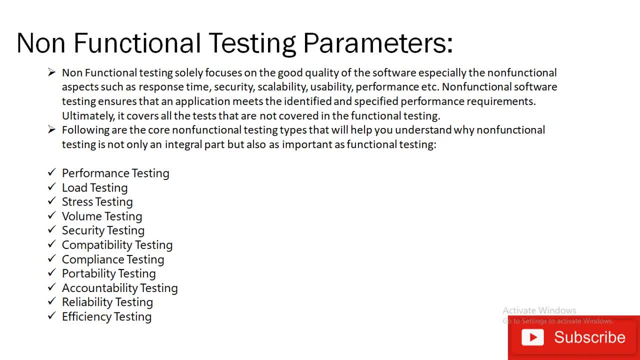 on their system. so that needs to be keep in mind while testing so compatibility in terms of browser, in terms of website. so if we are talking about any application, desktop application, and that desktop application is working in the some of the operating system and not working in other, 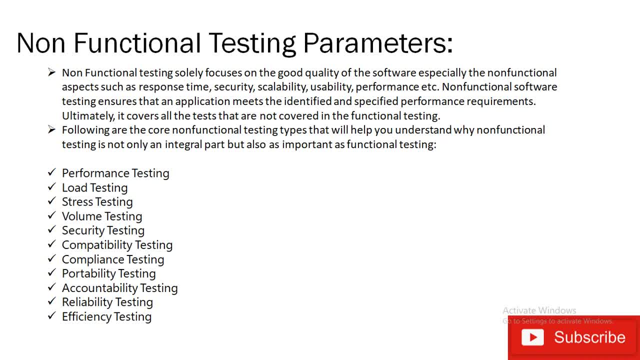 operating system. and just like if i am taking example of windows 7 and linux, so if i am launching that application in linux environment and same application is working for the windows only, so that is the compatibility in terms of operating system. so there are several other tensors also involved, so we will take one by one these parameters. so just like first parameter is: 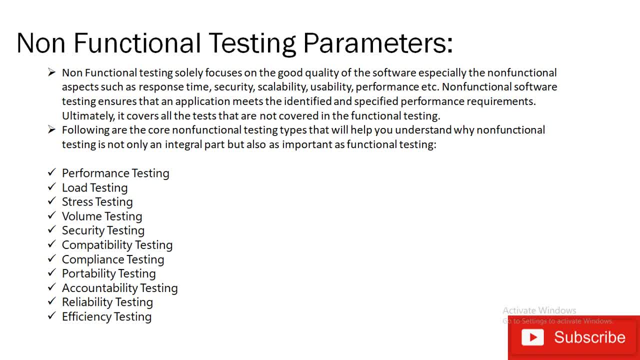 performance testing, so non-functional testing could be equivalent to performance testing, in addition to evaluate performance of the software it have in ensuring in response time aligns with desired time. just like i already explained in the beginning of that, just like if i am taking an example of the 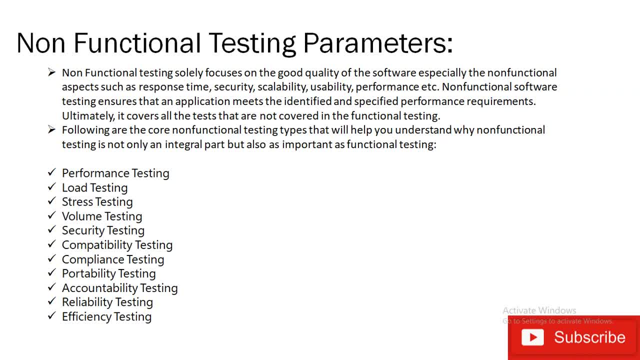 flip card application or admired website. so just like if I am the user I want to put just any of the product. like i want to post is any mobile application or mobile, the latest mobile launch in any of the brand. so just take an example: x1. i want to buy x1 as a mobile product, so i will select that. check the description while. 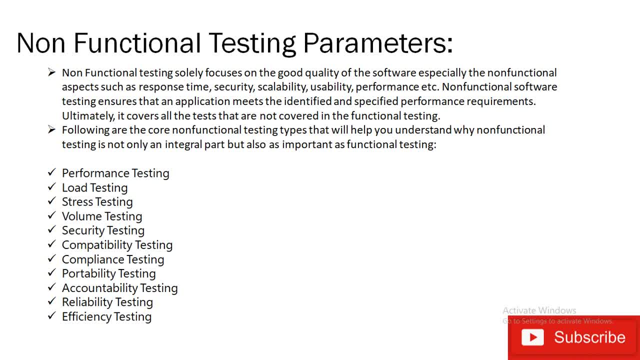 checking that description, performance should be clear, so i should get the response within 30 seconds in a time, just like i check the description. i want to add that product, or x1 product, in my cart, so while adding, it should add immediately, without a fraction of second. 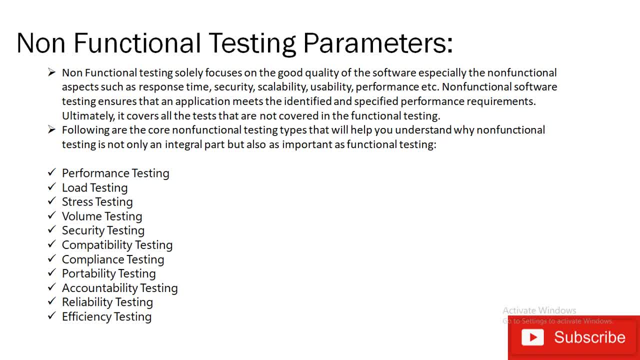 sorry, within a fraction of second after adding uh, that product in my cart, i want to buy that product and make a payment online. so when i'm selecting to buy should get enable that the product delivery location. so when i check that delivered location, it should immediately pop up for me as a payment option if i want to. 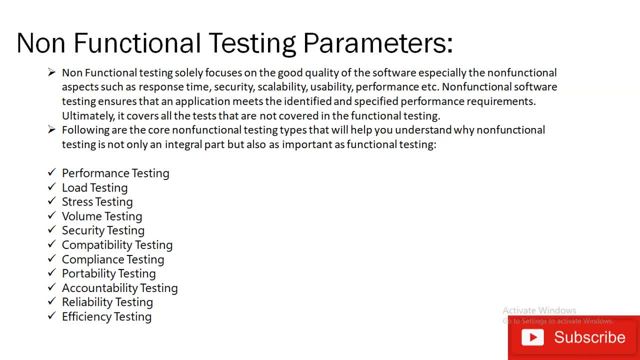 make a payment through online channel. so i should select um checkbox online payment. then i jumps to the payment method and i did the payment after entering all the details. so the performance should be as smooth as other websites. so, just like if you are taking any example of the mega sales offer, that time website is not properly working because of the millions of 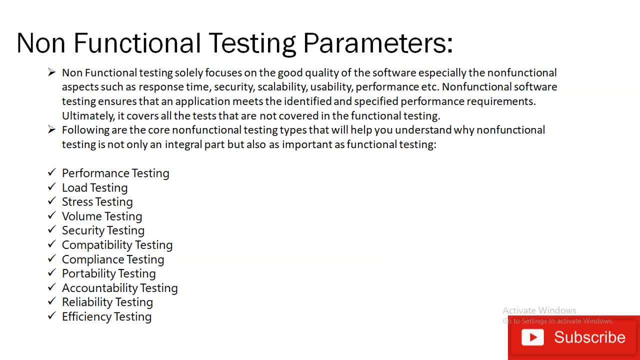 millions of customer is using same website in same product at a time. so for checking the load perspective, the performance and its response time should be clear. so here we are checking the start time, end time and the response we are getting after making request. so by setting up a considerable load and production size database, the application: 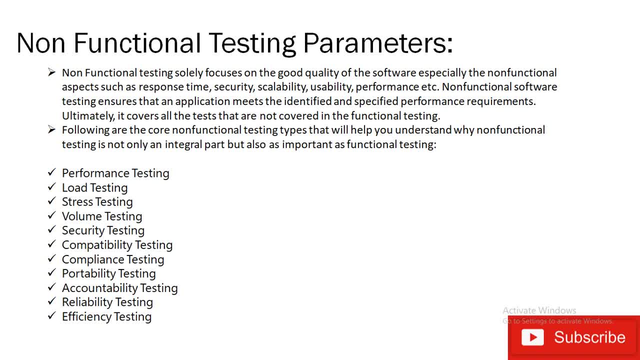 is tested for response time of several business critical processes. performance testing is carried out as a part of integration testing as well. so next is testing. so, as i already said, for the flipkart application, when mega sales offer are enabled, so that time that flipkart should work properly. so before going any application into production, 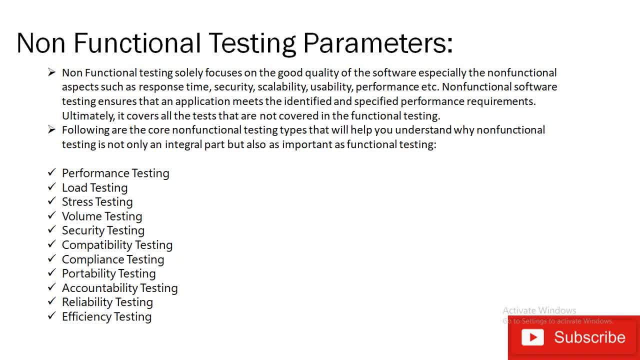 the testing team should check load testing as well with performance testing. so load testing is carried out to check whether the system can sustain the pressure or load of many users accessing the application at a time. The production load is replicated in the test environment to get the accurate results by loading load testing. 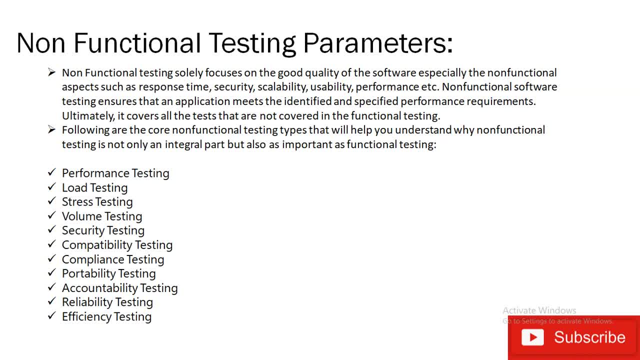 The same test is conducted, again in real time, with multiple users, to validate the results. While keeping the database realistic, the focus remains- and ensuring the desired response time, irrespective of the number of users. Next is stress testing. Stress testing is conducted to push the application beyond its capabilities to observe how it reacts. 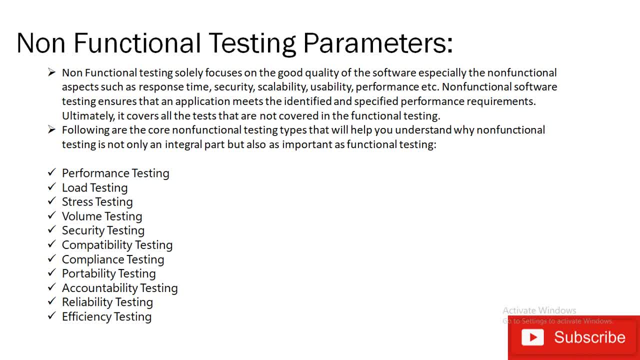 Contrary to load testing, where maximum capacity of load is generated, just like, if I want to test any website or login page sending the request of millions of users, 1 million users- that I will do that by using JMeter, So sending 1 million user request at the time of login at same time. 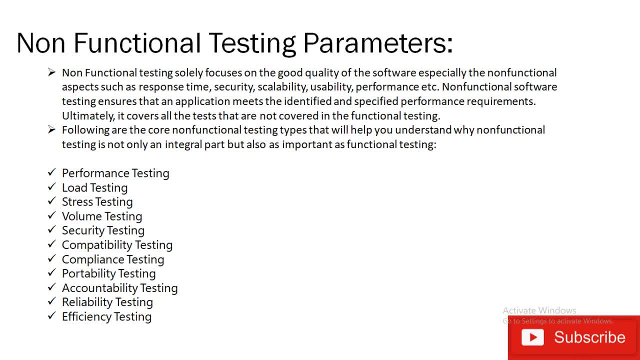 Stress testing is conducted where the load which is generated is more than the application can manage. Hence it is considered as an evaluation method of application performance in critical situations. Next is volume testing. Volume testing is carried out to check the storage requirements and capability of the application. 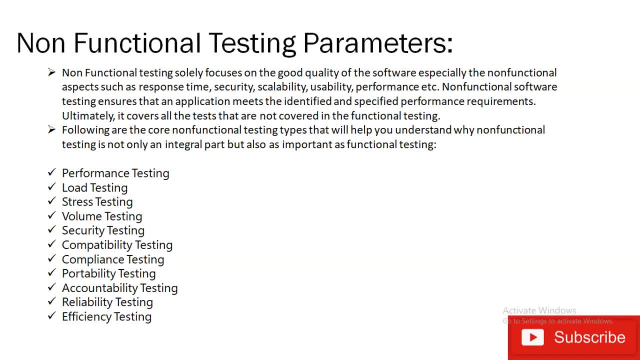 At times when the database is very large in size, Performance of the application and its ability to exchange data and And informations are tested with volume testings. So, as I have already explained about the compatibility testing, So compatibility in terms of OS, browser and several other components. 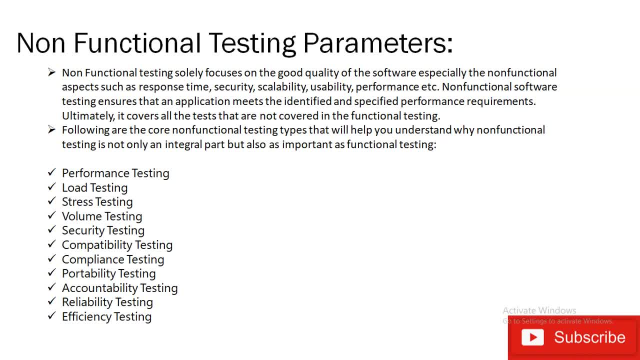 Next is security testing. So, while in my previous example, while making payment, So security is very important- role plays in a when we are working or doing a any payment, So that, in terms of finance, So the foremost requirement, even more than a smooth functioning of an application- security are implemented order to test how well the application can preserve itself and the data it holds in a situations of malicious attacks. 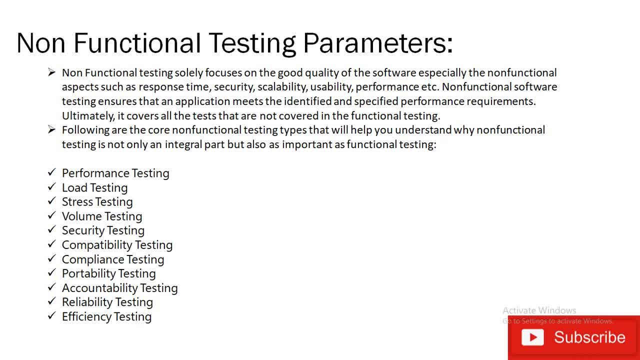 So confidentiality, integrity, availability, authentication and authorization are the key areas that are focused to be tested when security testing is conducted. In addition, network security, system security and application securities are areas to be focused on for the security of applications. Next is compliance testing. 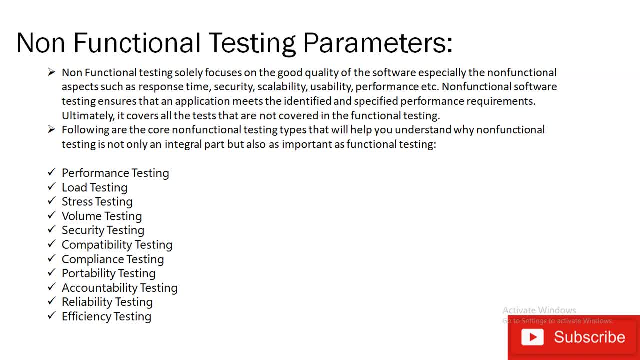 Compliance testing. we are testing the documentation part, its terms and conditions. Next is portability testing. So portability testing is basically done on the. that application is almost same as compatibility. So portability is a part of compatibility testing. So testing the ports and their applications. 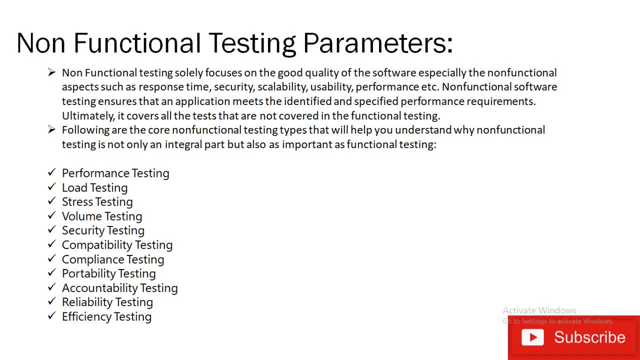 Other related components: Accountability testing. So in accountability testing, checking the desired or most specific accounts related information, Reliability testing- is the application is reliable to use to the user- is main questions while we are testing on the reliability Efficiency- is that application is efficient to handle? 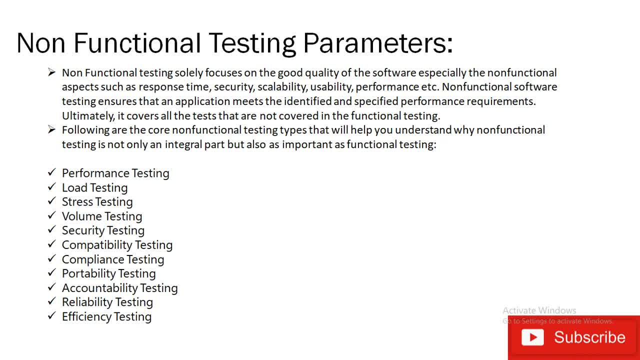 The millions of load at a time. So in terms of functionality, we can take example of login page when we are doing login on millions of subscriber at the same time, at the time of payment as well, at time of adding card, at the time of making payment. 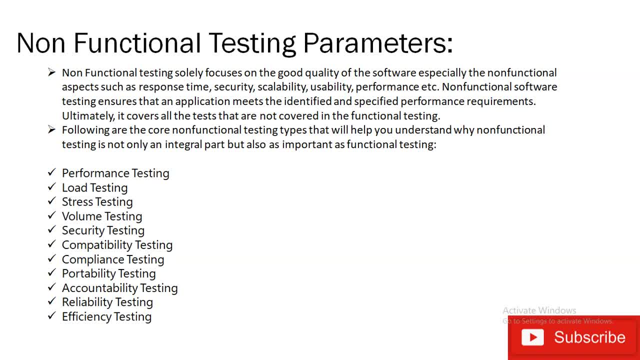 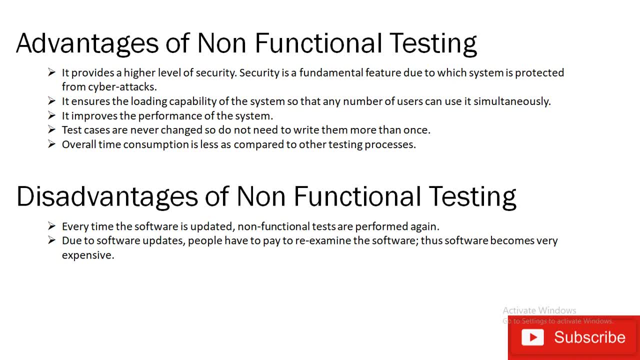 These all functionalities should be covered in the efficiency Now advantages and disadvantages of the non-functional testing. It provides A higher level of security. Security is a fundamental feature due to which system is protected from cyber attacks. It ensures that loading capability of the system so that any number of users can use it simultaneously. 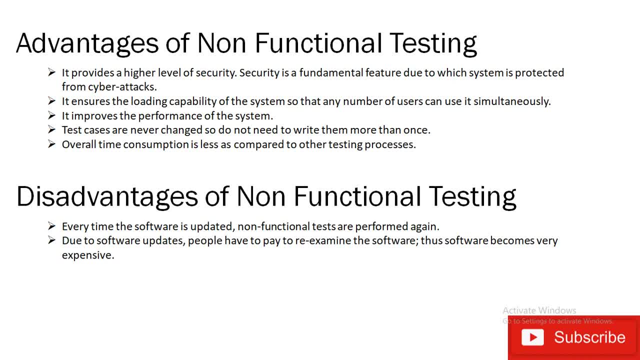 It improves the performance of the system. Test cases are never changed, So do not need to write them more than once. Overall time consumption is less as compared to the other testing processes. Now disadvantage: Every time the software is updated, non-functional tests are performed again due to software updates. 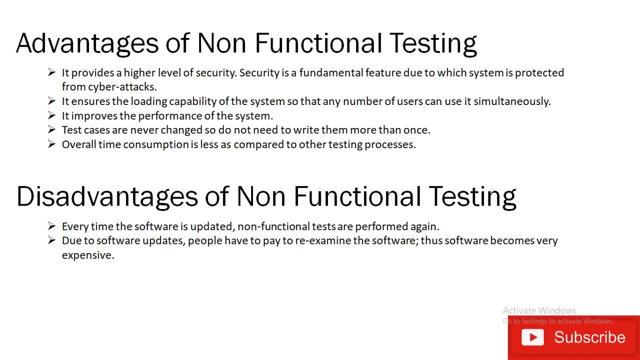 People have to pay to re-examine the software, The software becomes very expensive. So, apart from that, there is a failover testing, then usability testing, scalability testing is also a part of performance testing. So, first of all, what is failover testing? 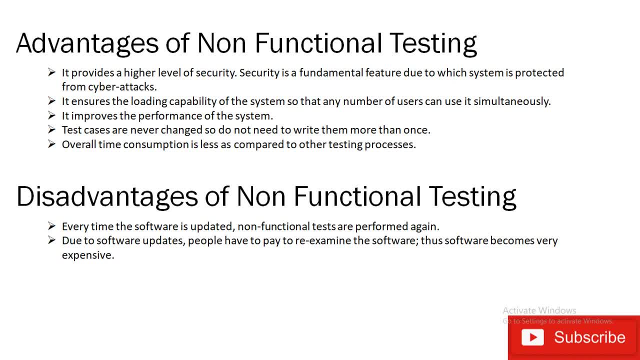 Failover testing has in understanding How the redundancy mechanism works when the system encounters heavy load or unexpected failure. Also, when the specific failed system is back again, it must begin to function as per requirement. Thus, failover testing is not only required but also important in the non-functional testing. 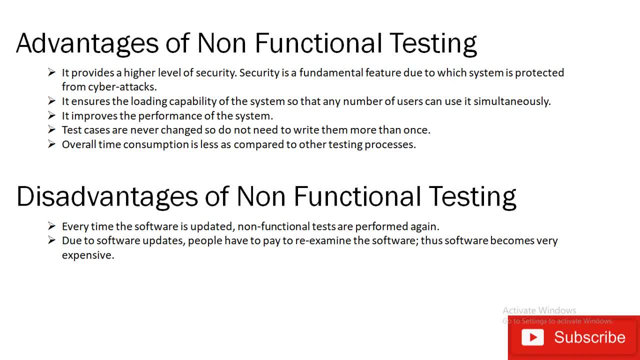 of the applications Usability testing. The purpose of usability testing is to verify the ease of software of an interface within an application. The focus area are learning ability and memorability of the application. Usability testing is extremely important, especially while testing the GUI. 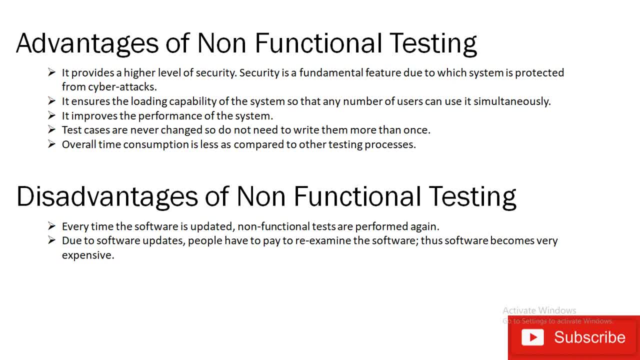 Scalability testing. Scalability test will help you to check the ability of an application to increase and scale up on any of the non-functionality requirements, such as load, number of transactions, number of servers, volume of data, etc. When there are no non-functional applications. 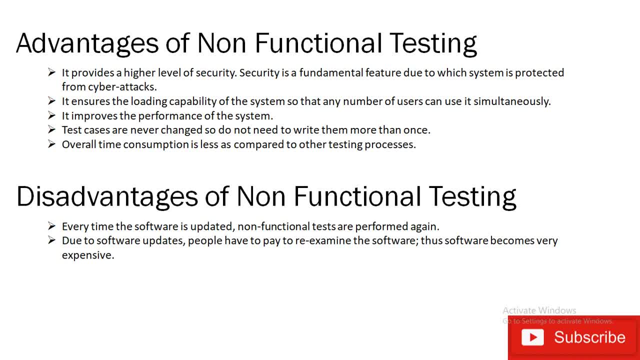 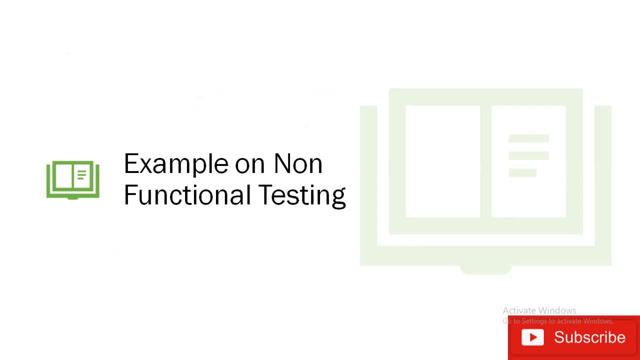 When there are no non-functional applications, When there are numerous tests exist, including functional and non-functional. we have shortlisted and explained the most important ones in this session. So this is all about the advantages and disadvantages and their parameters. Let's take one example again. 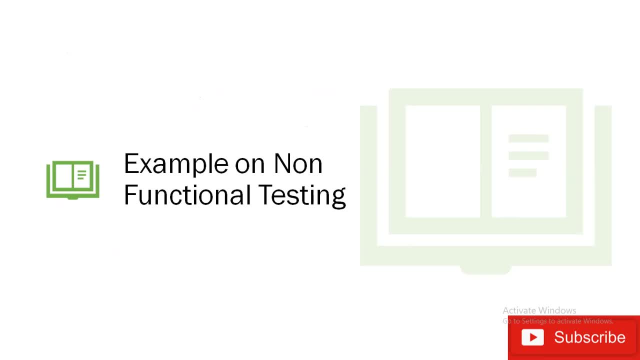 So, just like I have already explained about the Flipkart application, I am taking one desktop application or mobile application, Just like we are considering example of WhatsApp application. So let's take one example, Just like we are considering example of WhatsApp application. 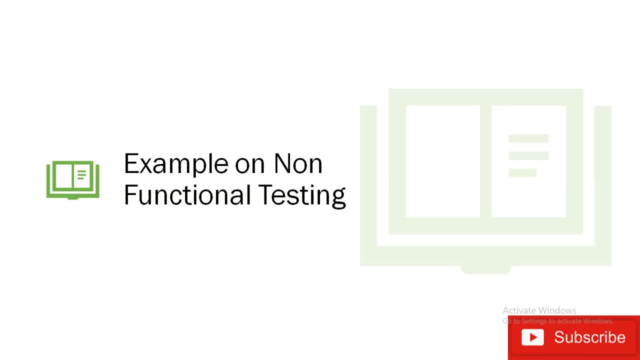 WhatsApp application is mostly used in all of the country, So when we are talking about the message perspective, when several matches incoming or several matches sending together, the performance of application should be seen as when we are sending for this single user, So that testing should be done before application goes to the productions. 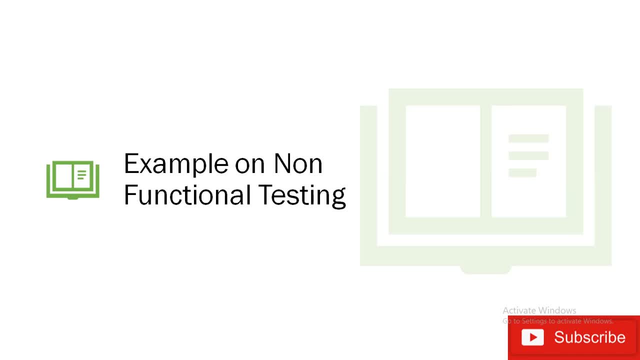 So same idea thing also happen when we are doing a single call, a video call with one-to-one basis, and when we are having a video call with multiple user. the performance should be same in both the cases. so that should be in mind while testing this, these type of applications. so just like, if you. 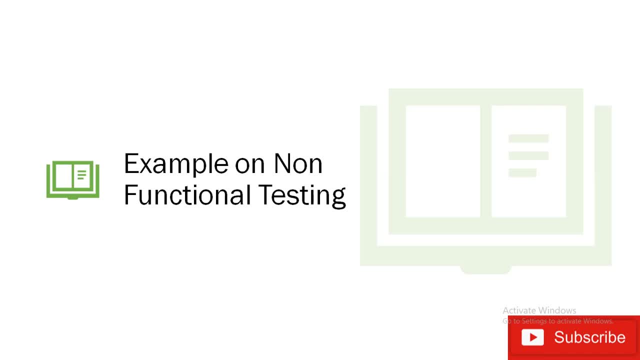 are taking an example of the login page and there are 10 000 plus users are logging at the same time, so the application performance should not go down. so response time should be almost same or there should be a negligible differences when we are doing login for one user and when we 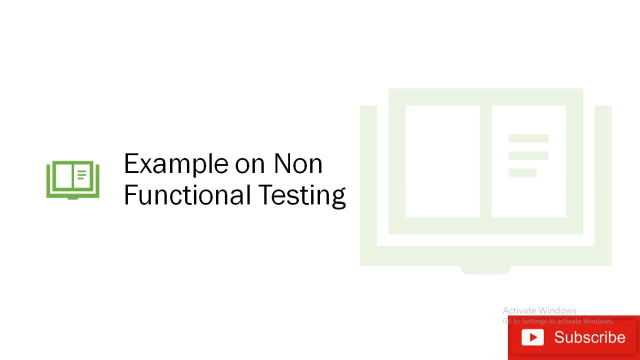 are doing 10 000 plus user, so this is a mid-range application. we are talking about that, but when we are talking about the high range application like flipkart, amazon, gmail, so these type application performance should be always be in the higher side because these applications are regularly used by the worldwide. so these are the examples of the 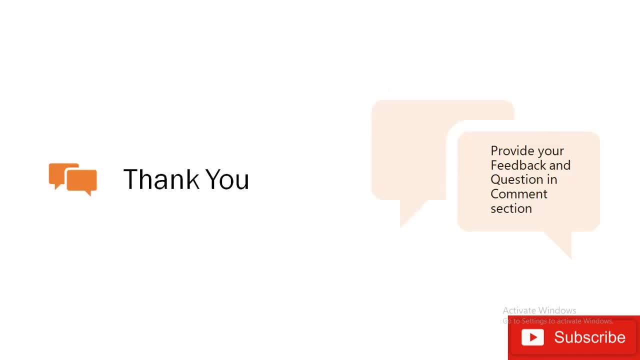 non-functional testing. now we have this done about the non-functional testing. hope you understand it. if you have any queries or comment, please comment in the comment box so that i will check and reward you for this video and i will see you in the next video.